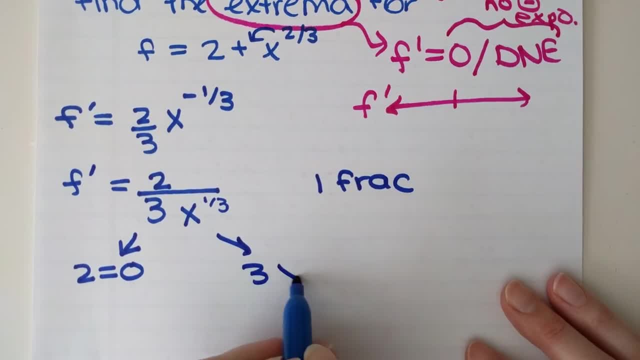 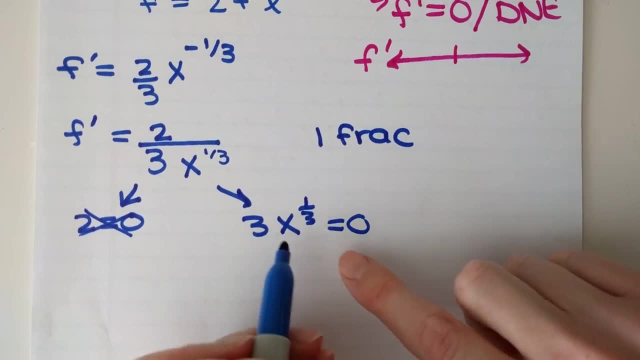 so 2 is equal to 0, and the denominator equal to 0,. 3x to the 1 third is equal to 0.. Now, from 2 is equal to 0, we get absolutely no information Over here. you could just say that x is equal to 0, and the reason for that is because if you divide by 3,, 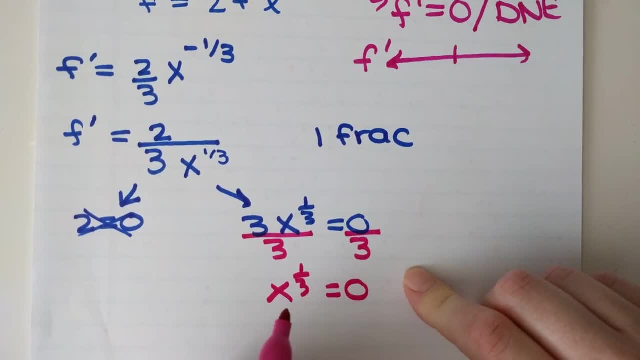 you are going to get x to the 1 third is equal to 0. Then to undo this 1 third, we're going to have x to the 1 third and then to undo this 1 third power, we would raise both sides to the reciprocal. 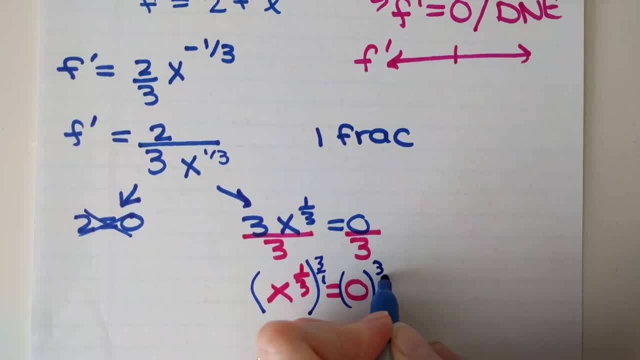 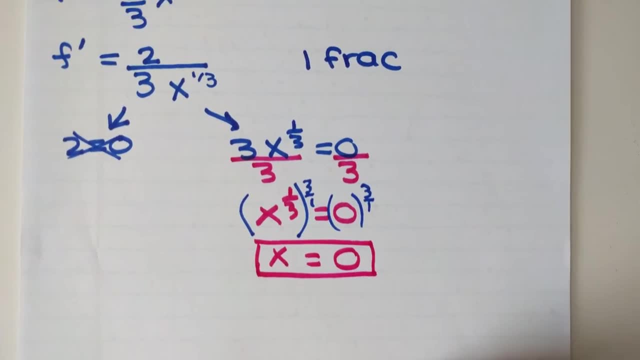 which would be 3 over 1.. But if you raise 0 to the 3 over 1 power, you just get 0. So you are going to get: x is equal to 0. Alright, so with that critical number we then draw our number line. 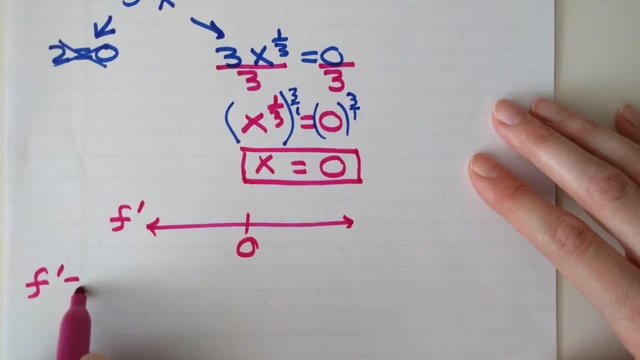 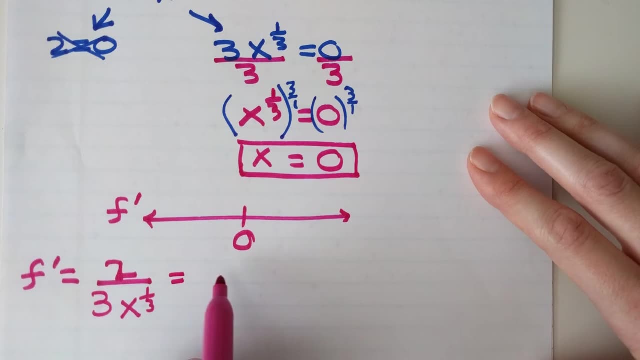 And it's probably easiest if you work with the one fraction derivative. So we had 2 thirds x to the 1 third power, Alright, so keep in mind that this is the same thing as the cube root of x. So you can use your scientific calculator to plug in a number here. 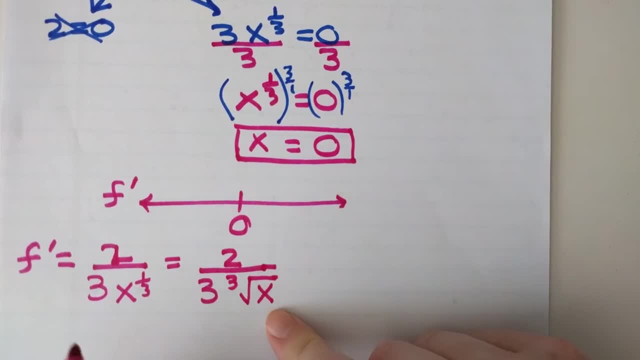 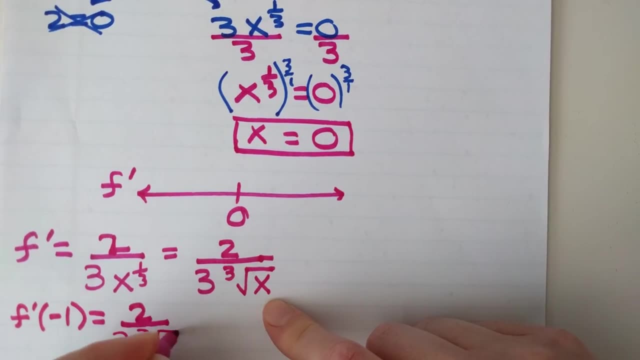 but you just have to have some way of figuring out the sign. So, for example, if I plug in negative 1, I am going to have 2 over 3 to the cube root of negative 1.. And the cube root of negative 1 gives us a negative. 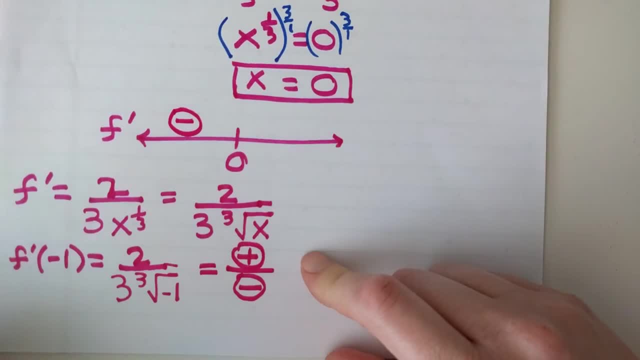 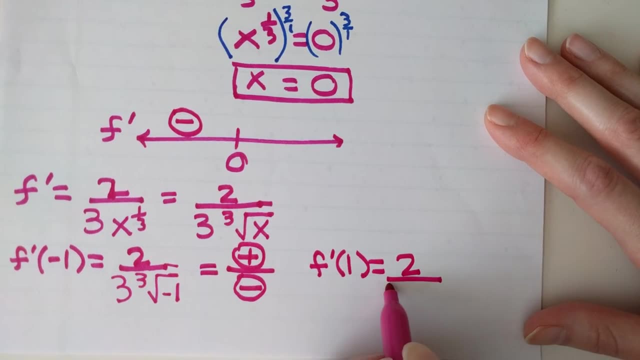 so we have a positive over a negative and so we just get a negative. Now, if I plug in a number to the right in the square root of 0, let's say I plug in 1, in that case I have 2 over 3 cube root of 1,. 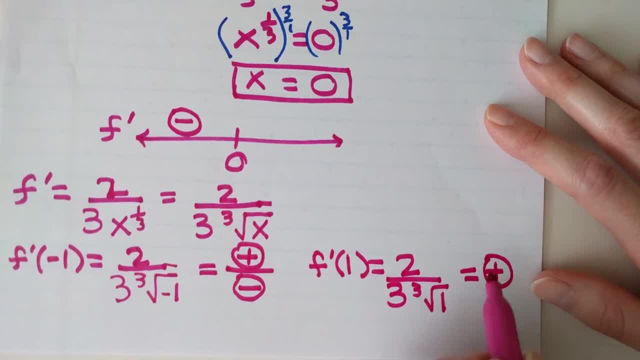 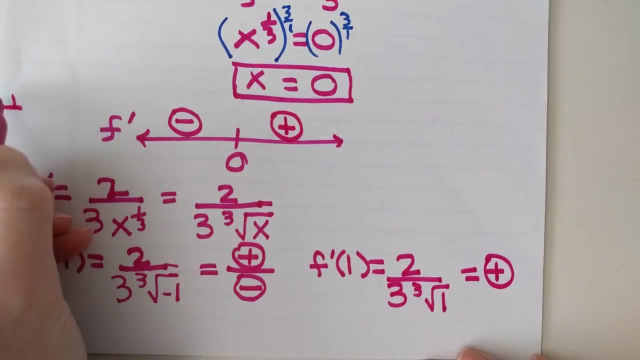 and there there is not a negative in sight. so that is going to evaluate to positive. So we have a positive, Alright. so looking at our number line, remember: 1st derivative tells us increasing and decreasing. So this negative tells us that we are decreasing until 0,. 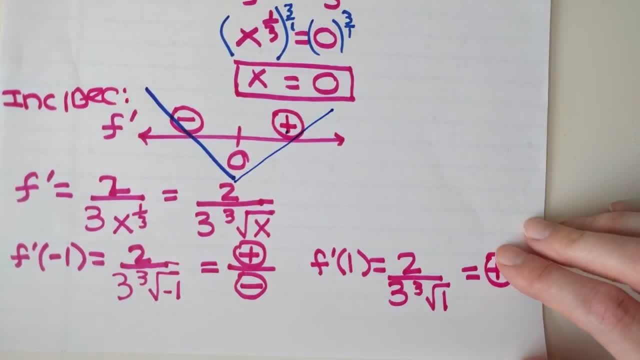 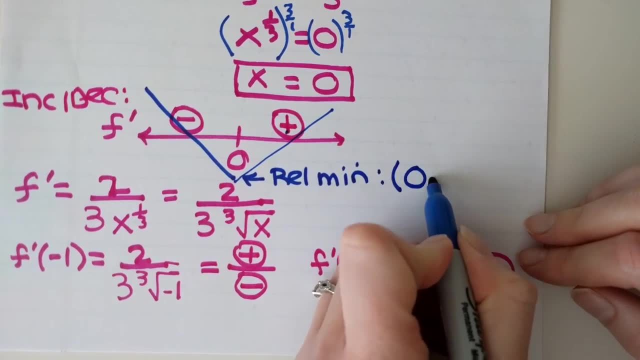 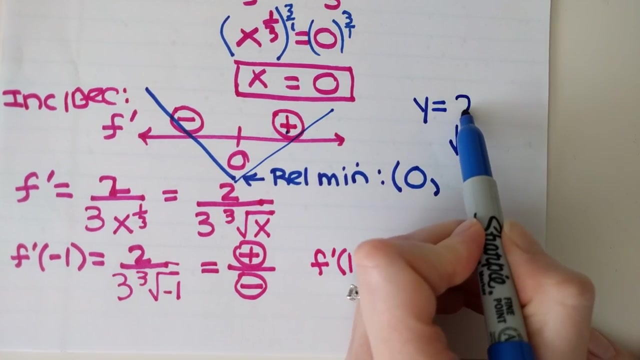 and this positive tells us that we are increasing after 0. So 0 will be a relative min for us. Now to find the corresponding y value you need to plug it into the original function, the original y. So our original y was 2 plus x to the two-thirds. so plugging in 0, we will.